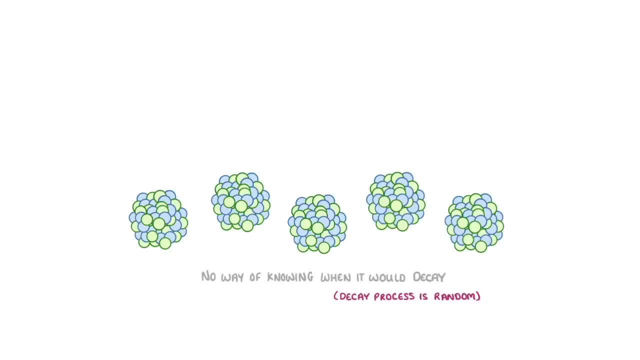 still find out two very useful things. One is the activity of the sample, which is the overall rate of decay of all the isotopes in our sample. and we measure activity in becquerels, where 1 becquerel represents 1 decay per second. So if a sample had an activity, of 600衹 M, then we'd be able to Randolph, Thereby find values subject to an sparkle or Woolei boson hardness. Then, of course, once we missed, we would work on71 to use 12衹 M and puzzle is drawn to the appropriate depth, We would calculate the rate of the 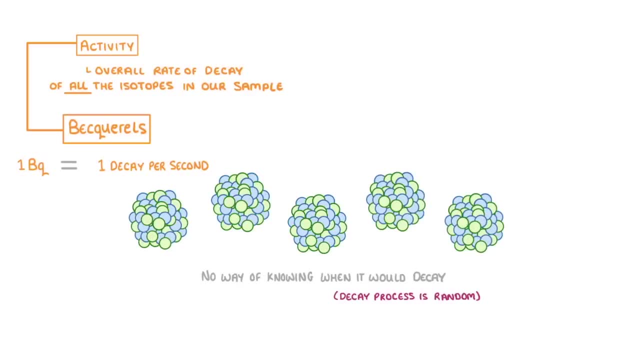 100 becquerels, then there must be 600 isotopes decaying each second in that sample. The other important term to know is half-life, which has two definitions and can be defined either as the time taken for the number of radioactive nuclei in a sample to half for 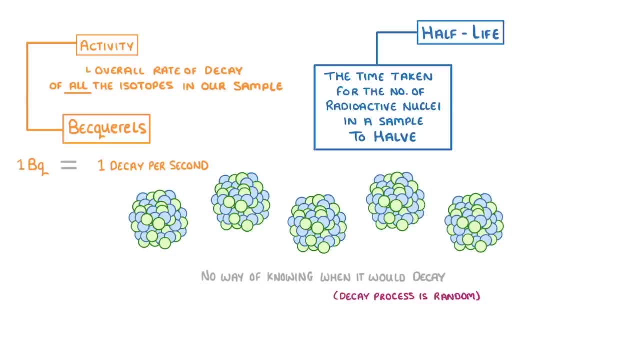 example, to drop from a million unstable nuclei to only 500,000, or the time taken for the number of decays, so the activity to half. for example, to drop from 600 decays per second to 300 decays per second. 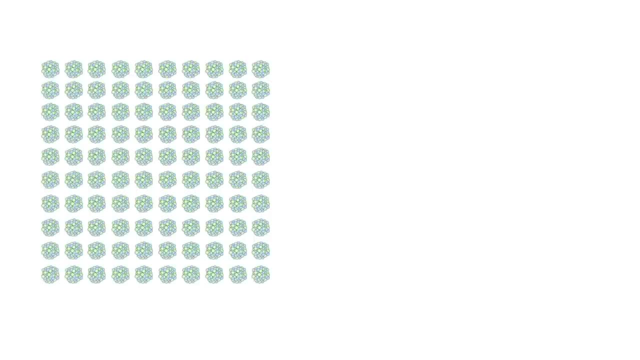 To properly understand these concepts, let's imagine our radioactive sample as 100 unstable isotopes, each of which can decay by emitting radiation in order to become stable. So if we watch this sample decay, The first thing we notice is that the decay process is completely random, so we have no 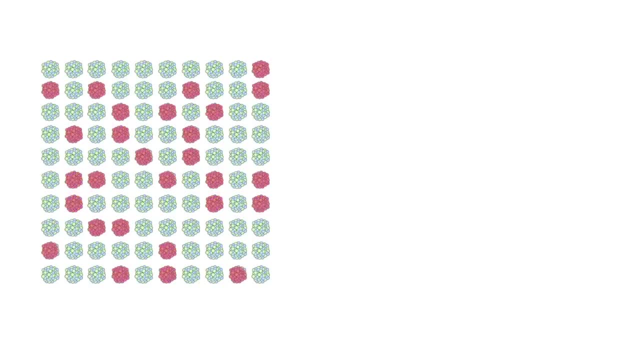 way of knowing when any particular particle will decay. As time goes on, though, and more and more of them decay, the number of unstable particles remaining decreases, Because there are fewer particles left to decay. this means that the overall rate of decay- which, remember, is the activity- will also decrease, which is why it looks like. 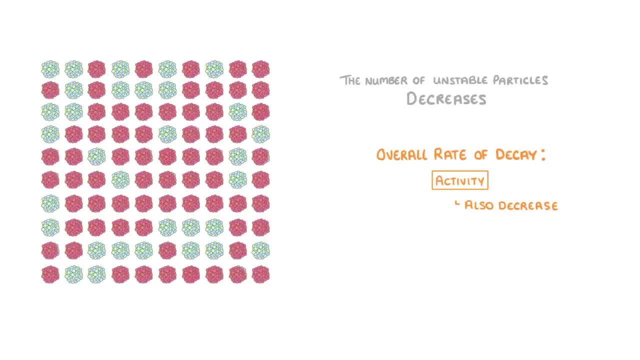 the sample is decaying more slowly than it was at the start. This is why we can define half-life as a halving of either the number of radioactive nuclei remaining or a halving of the activity. They are both perfectly correlated, because fewer radioactive nuclei means a lower activity. 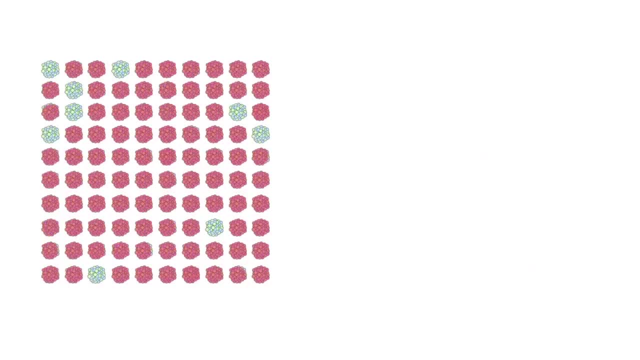 Another way to show this decay process is by using a graph that plots activity in becquerels against time. As time goes on, the number of particles remaining and the activity of the sample will decline, But the rate of decline will also fall, which is why it's curved rather than a straight. 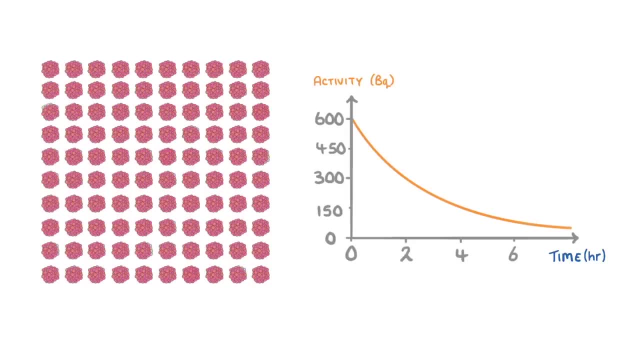 line. To calculate the half-life from a graph like this, we need to find the time it takes for the activity to half, So in this case, drop from 600 to 300, which we can see is about 2 hours. And to confirm this we could check another one by seeing how long it takes it to half. 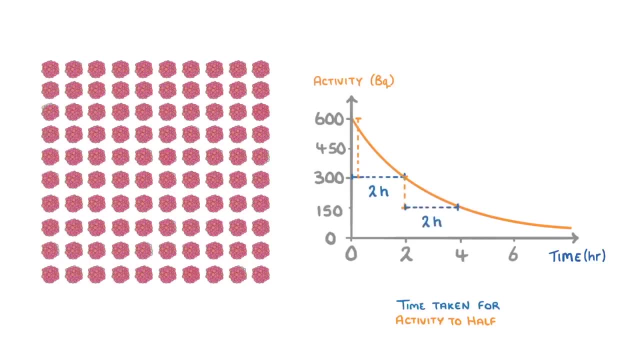 again down to 150.. And indeed it does take another 2 hours, so we can be confident that the half-life is 2 hours. If we had a different radioactive sample, though, like this one, We can see that it's decaying much more quickly. 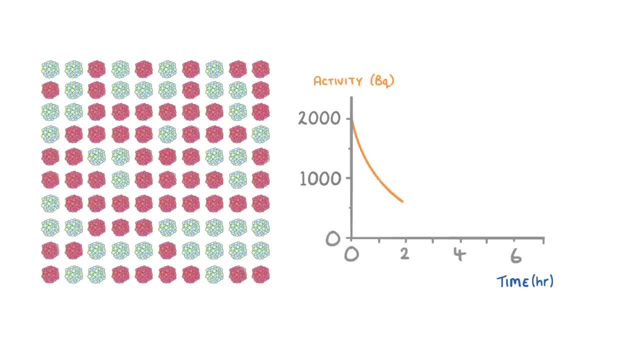 This means that it started with a much higher activity, as we can see on our graph, And also that it will decline much more rapidly and so a much shorter half-life. This time of 1 hour Now, so far we've just kind of assumed that we'd know what the activity is. 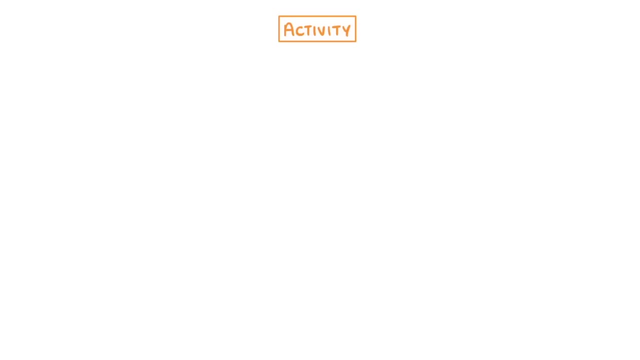 In real life, though, We'd have to find the activity using a device called a Geiger-Müller tube and counter These things, record all the decays that reach them each second, So all of those alpha and beta particles and gamma rays. 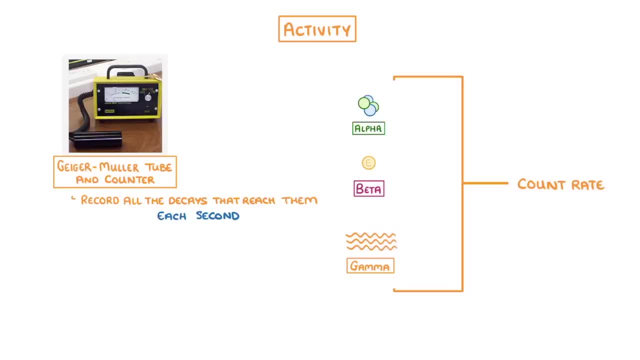 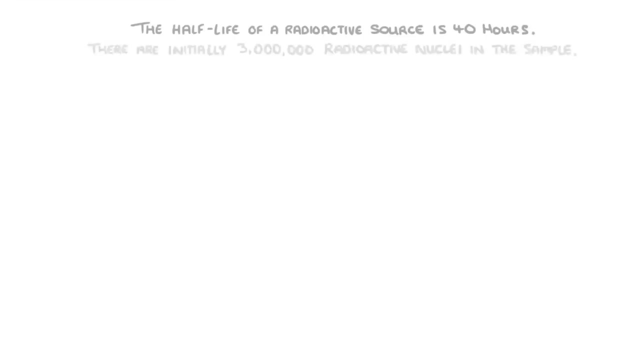 Which it then records as the count rate, And it's this count rate that we use to estimate the activity. Before we finish, let's try one quick question. The half-life of a radioactive source is 40 hours. There are initially 3 million radioactive nuclei in the sample. 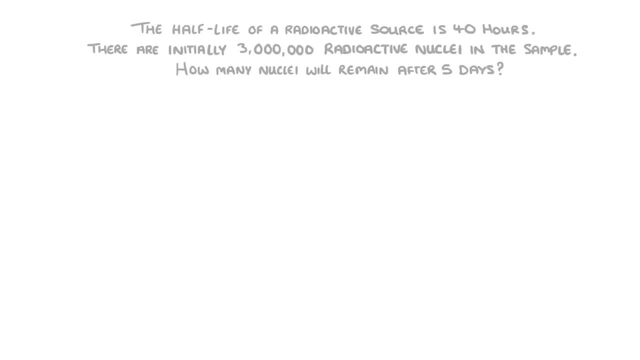 How many nuclei will remain after 5 days? In a question like this, the idea is to first find out how many half-lives there'll be And then half the number of radioactive nuclei that many times. So first we need to take 5 days.